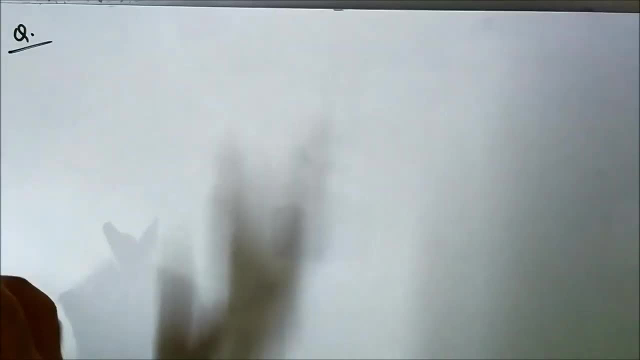 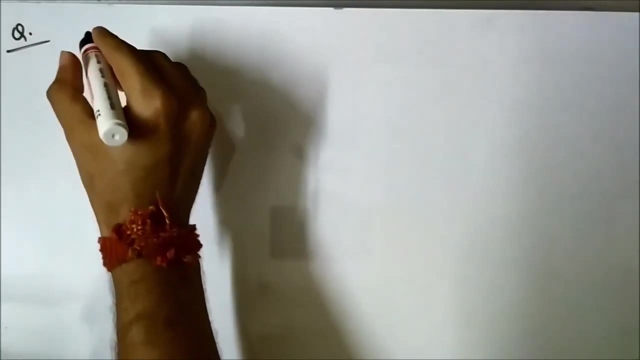 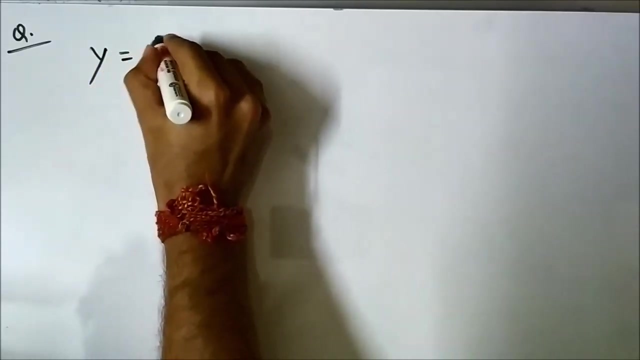 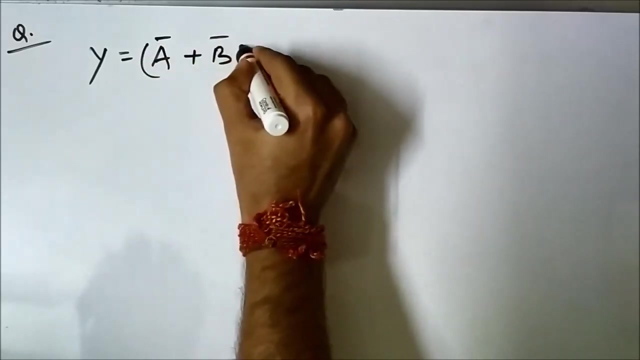 first question Is: to design a digital logic gate or combination of logic gates to which gives us this output. Ok, So we have to arrange another internal logic threshold, rather than I build a rats zone. So this one is: we have to figure out that we want an internal logic system for digital. 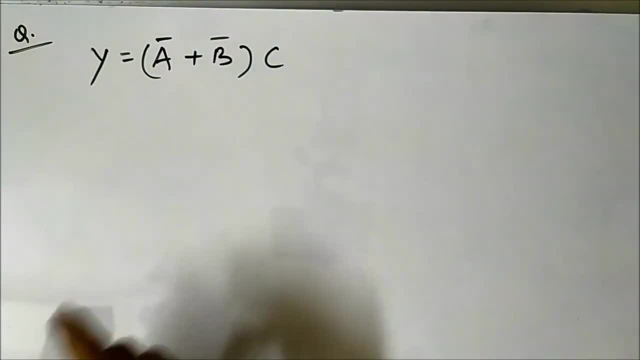 logic gate- number of digital logic gates, in such a way that the final output is this: now, whenever we come across any digital expression, boolean expression, and we have to design a logic gate for that, first we have to identify what operations- boolean operations- are there present in that expression. 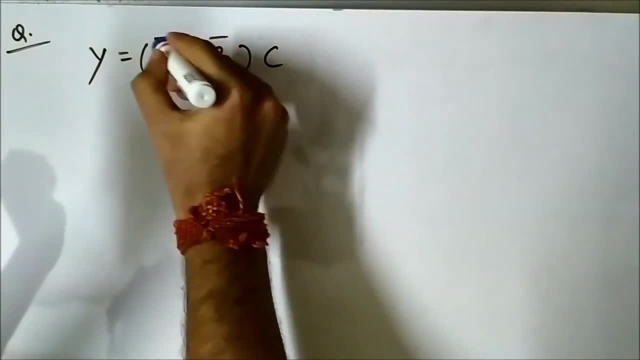 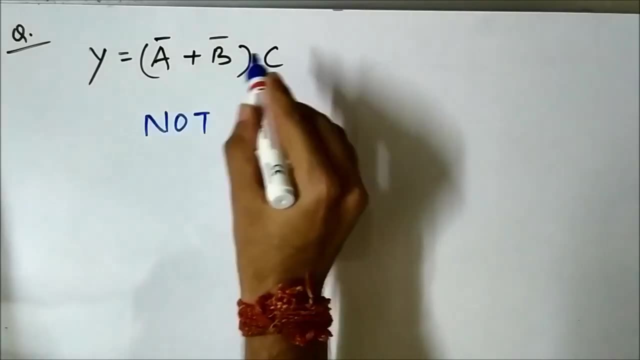 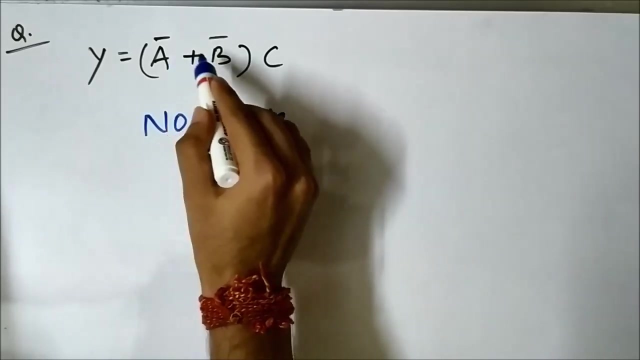 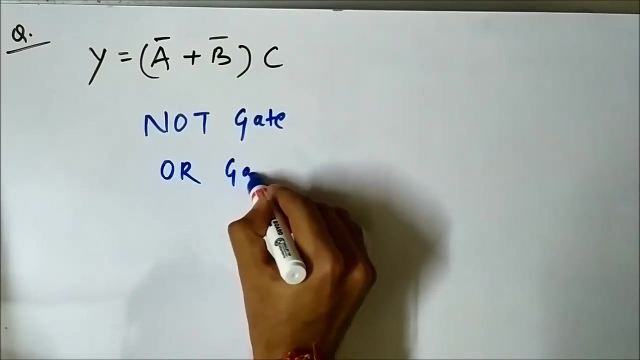 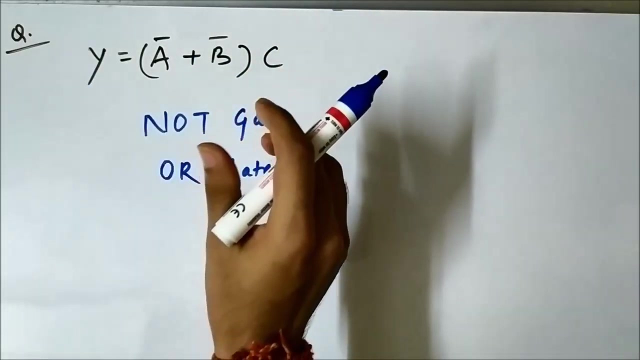 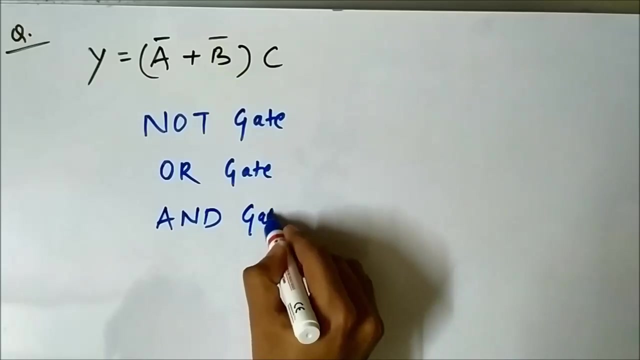 so here the bar on top of a and b. it represents not gate, because inversion operation is performed, so we require not gate. this plus sign: it represents or operation, so we will require or gate. and this the multiplication. in digitalization domain, it is the AND operation, so we will require a AND gate. so I have 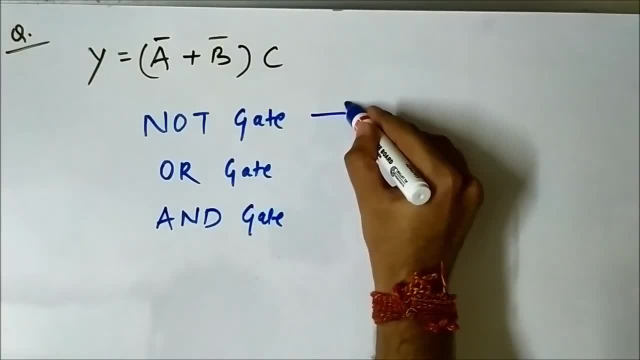 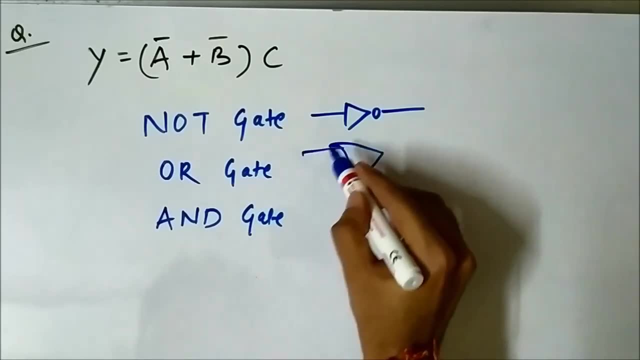 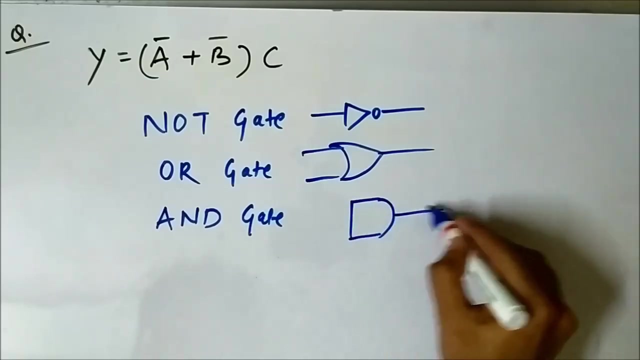 already discussed about these gates. so the NOT gate, it looks something like this, the OR gate, it looks something like this, and the AND gate, it looks something like this. okay, so we will use the combination of these three gates to give us this logic output. I have already discussed them about in detail, so you 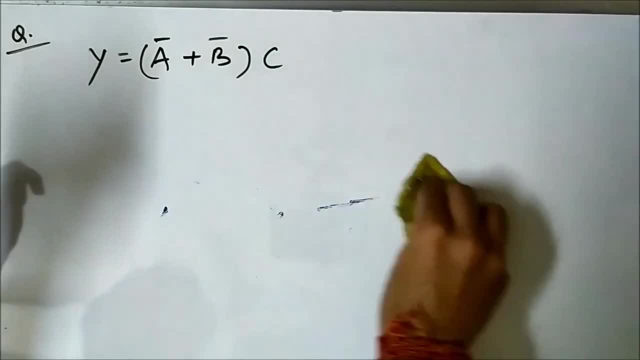 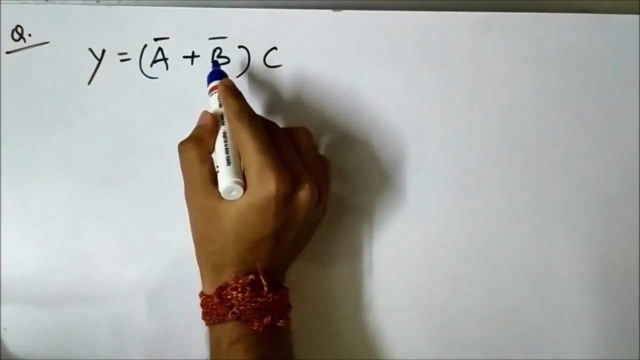 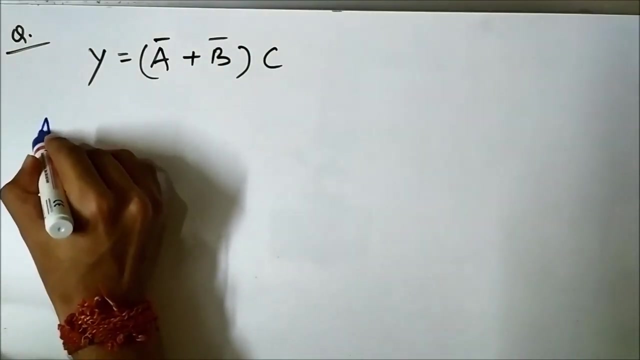 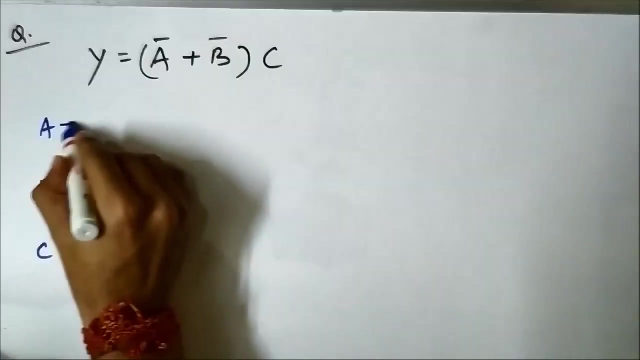 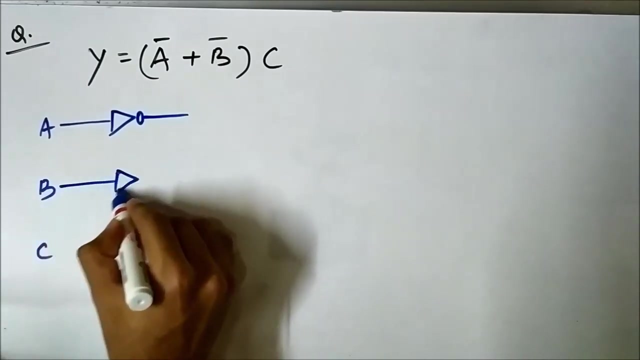 check out those videos. okay, so first, the signal values here are A, B and C. three signal values are present, so let us assign this them A, B and C. now A bar. for A bar, we have to pass it through a, NOT gate or inverter, same for B. so we got A bar and P bar. now we have to get this A bar plus. 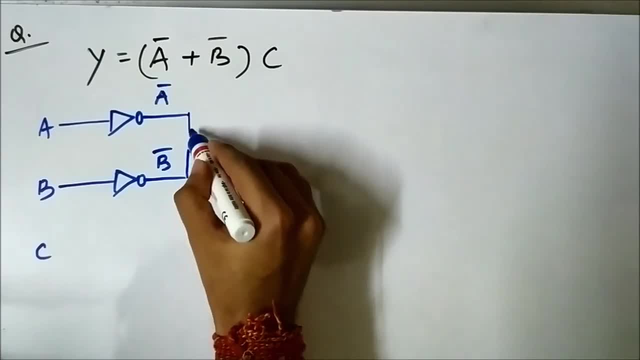 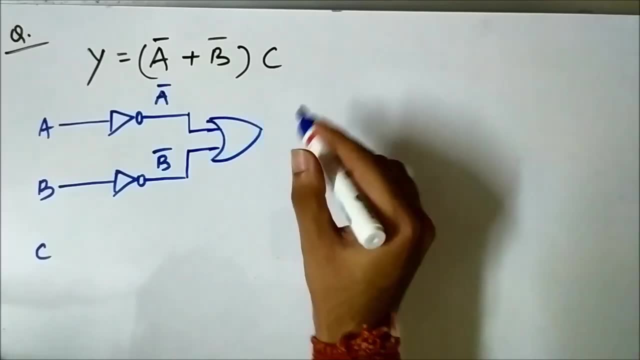 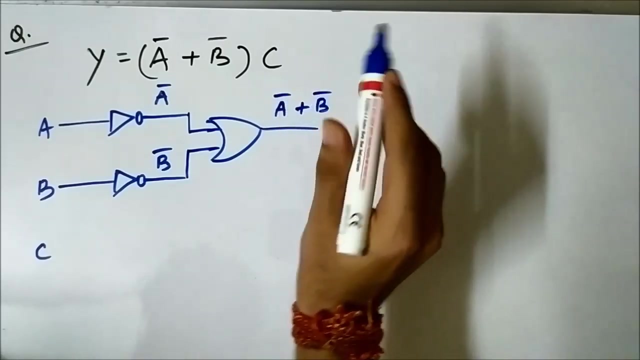 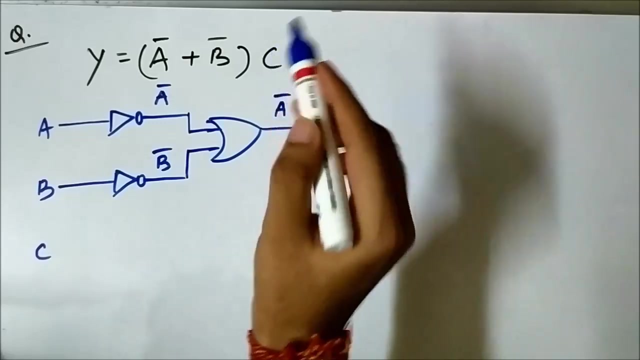 B bar. so we have to pass them through both these signals, through a OR gate. This will give us a bar plus b bar. Now again, I will repeat: when I say plus, it means a bar or b bar. When I say into or multiplication, it means that and that. 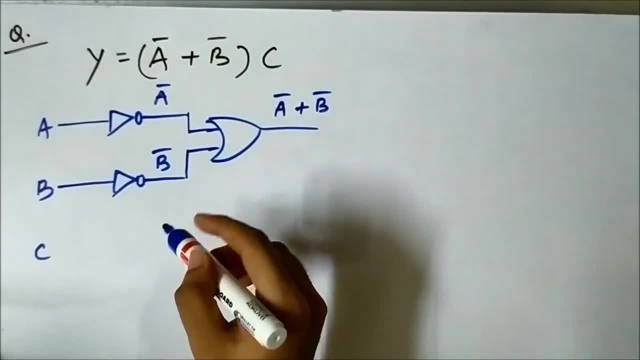 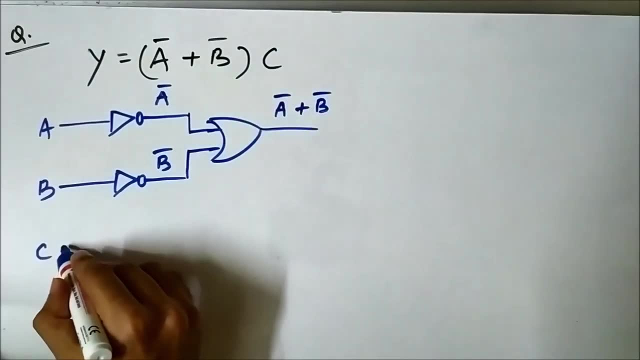 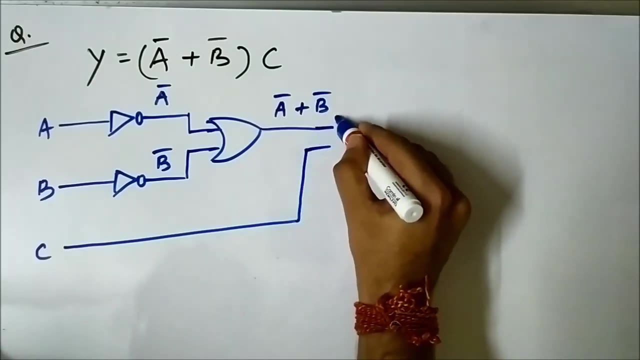 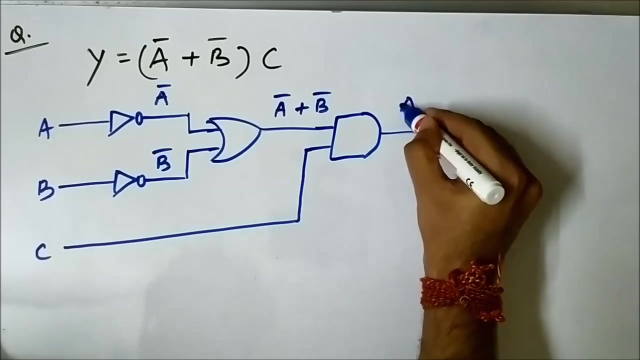 that means and operation and bar means not operation. Now we require this: a bar plus b bar into c or and c. So we have the c here and we have this here. So we will give them to a, to input and gate, which will give us a bar or b bar, whole and 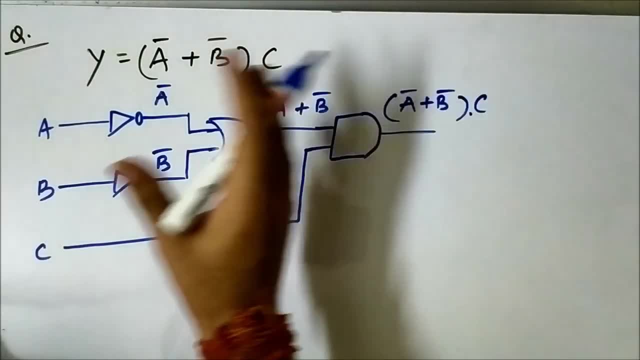 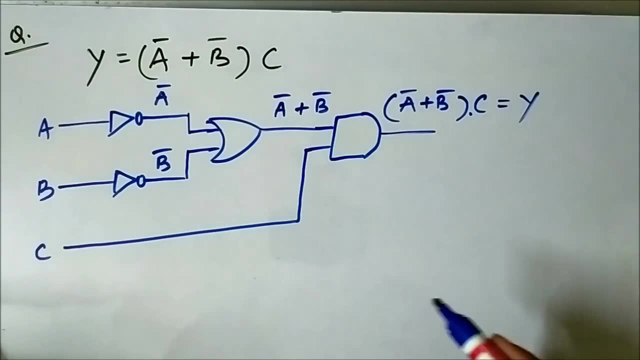 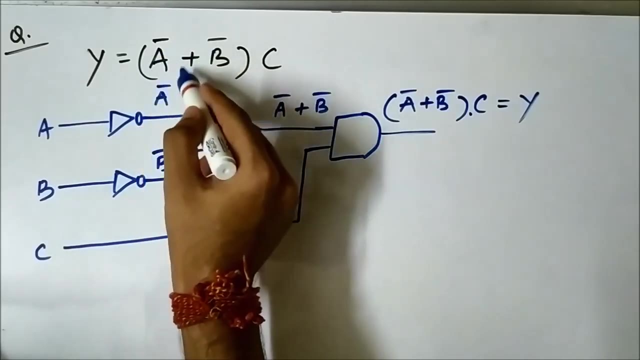 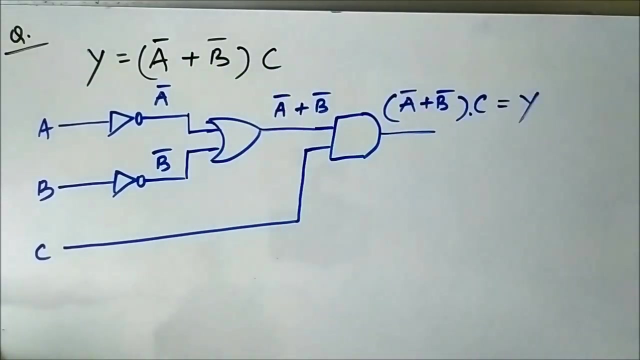 c. So this is the final logic output we got here. We got this output is equal to y, the final logic output. So we got these individual terms- a bar, b, bar, then we OR them together, then we added them- this signal and this signal- and we got the final output. 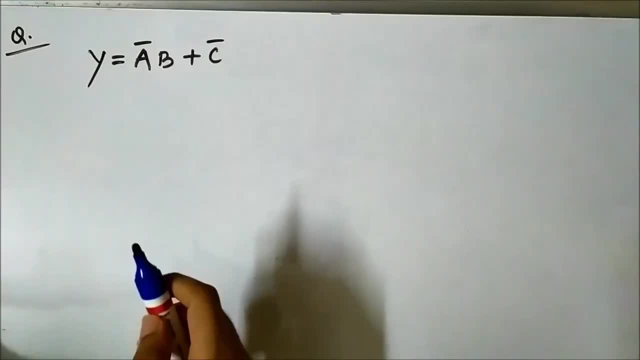 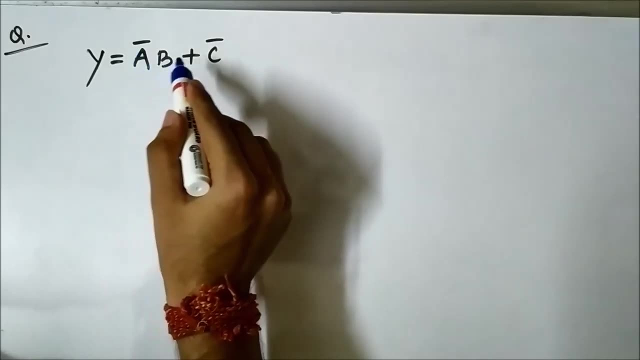 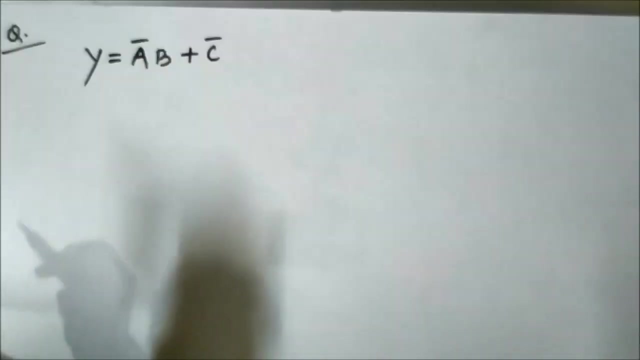 So here we have another expression which we have to implement. again we are taking a simple one which is again here. the expression is a bar b plus c bar, OR a bar b OR c bar. c bar means not operation. So again here the 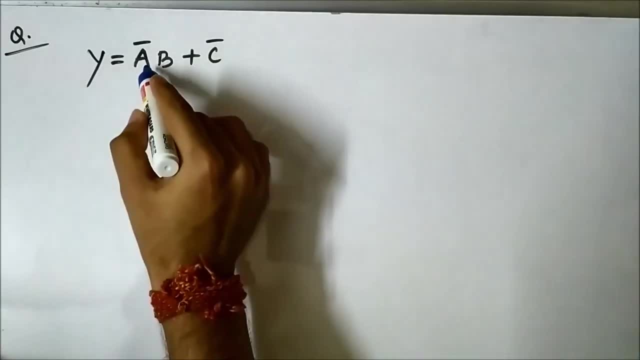 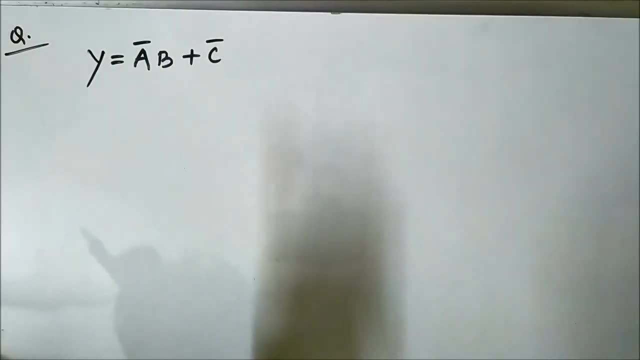 bar represents, will require a, NOT gate, or inverter. this AND operation between a bar and b represents will require a AND gate. and this plus sign it represents OR operation. So we require OR gate, NOT AND and OR. these are the three logic gates that we require. 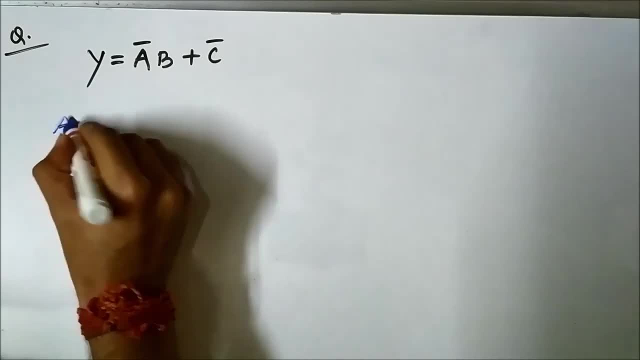 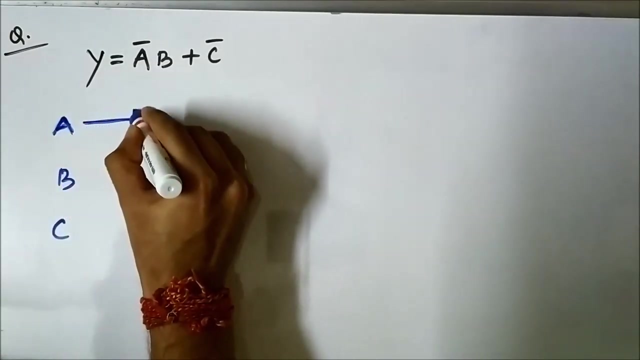 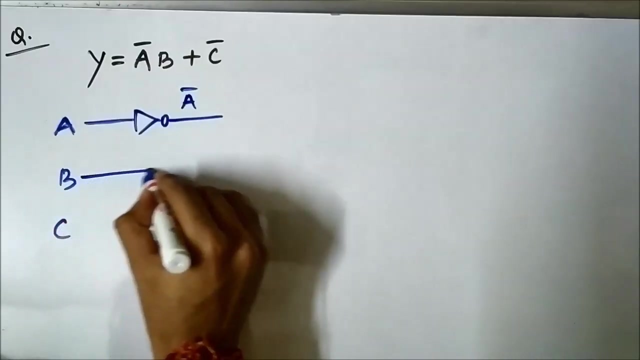 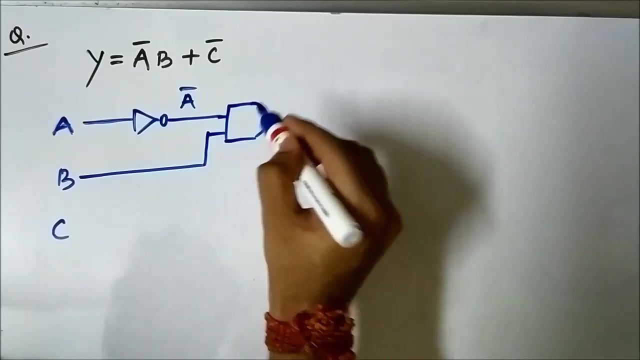 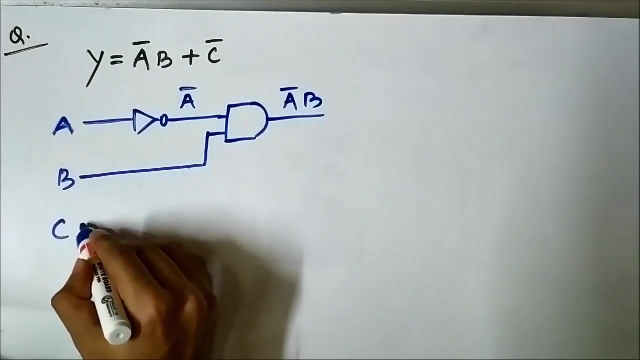 So first let us assign the signals a, b, c. Now we need first a bar, So we will pass it through inverter. we will get a bar, a, bar, b. for that we have to pass them through a AND gate, Which will give us a bar b, then c bar that we have to pass it through. 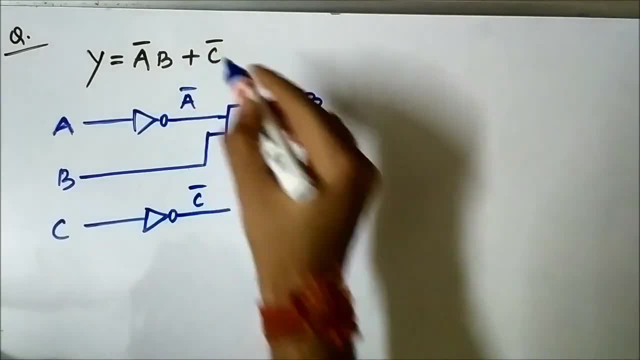 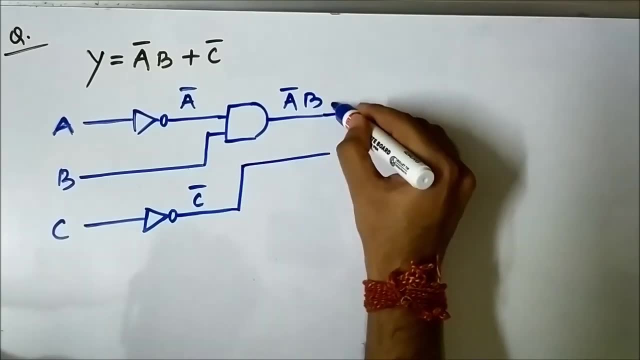 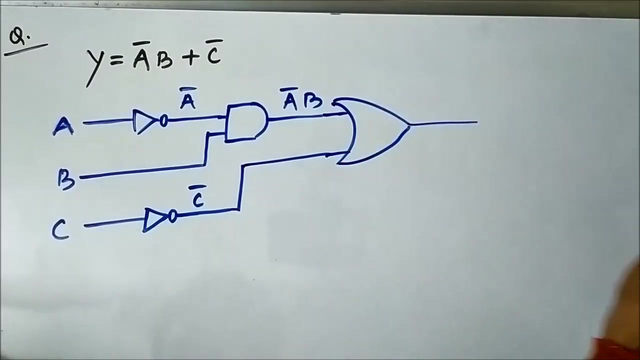 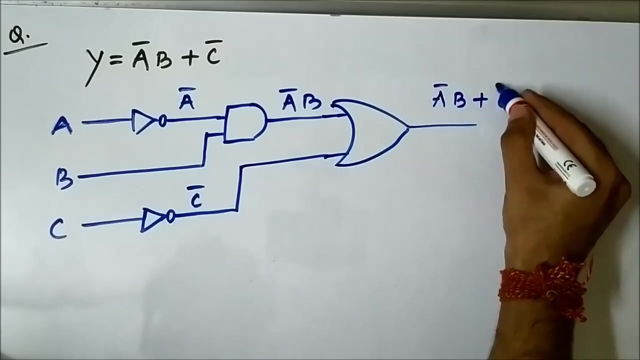 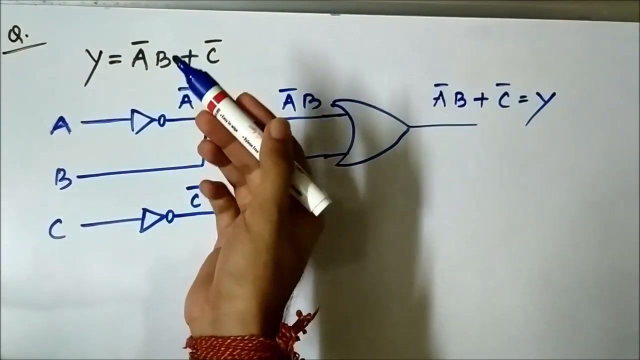 a, NOT gate, which will get c bar. then the OR operation between these two signals or the OR gate. So finally we get A bar, B OR C bar. this is the final output. So again the same steps. first we have to determine what logic gates are required. then we have 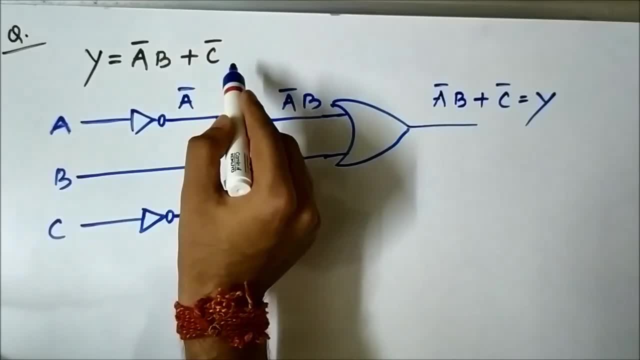 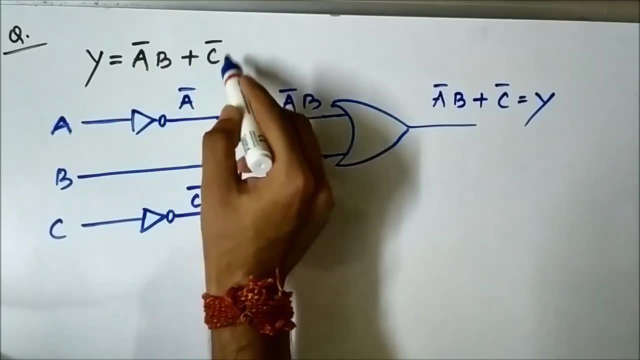 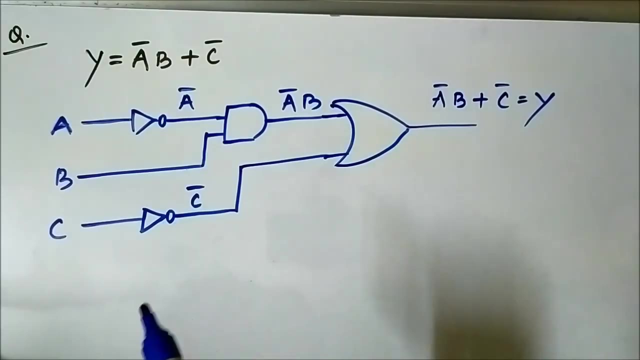 to target the individual terms that are present. how to get those terms first, For example, here: first we have to get the term A, bar B. we got it. So it is a simple thing, simple expression. that is why it was easy. we will move on to more complex and complicated expressions. 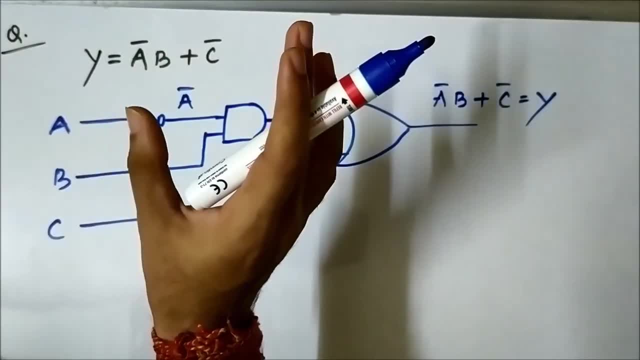 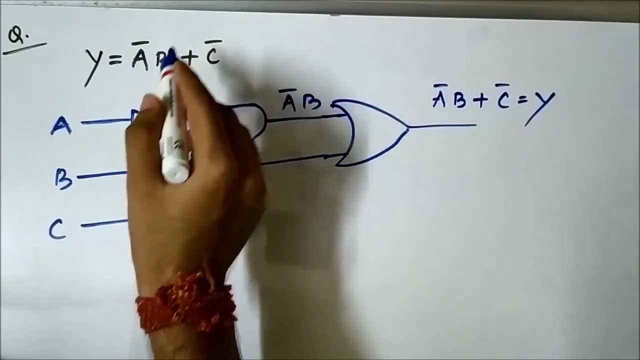 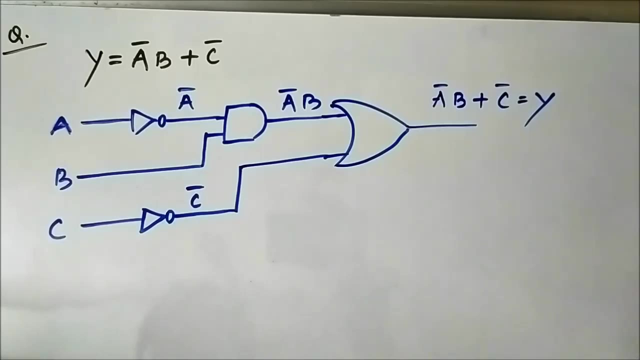 So first we have to determine what logic gates are required, then we have to create the individual terms that are present in the expression, Then we have to get the final expression. So here we have solved another simple logic expression using digital logic gates. we created the, we got the output.